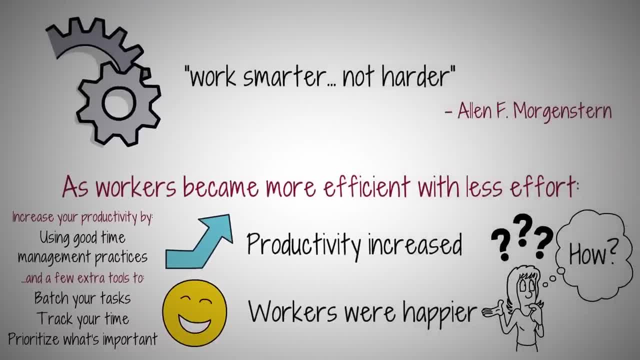 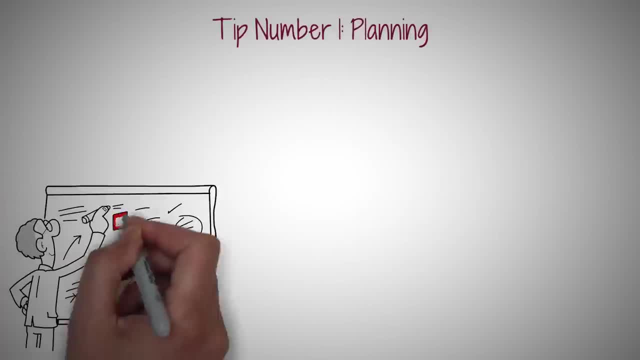 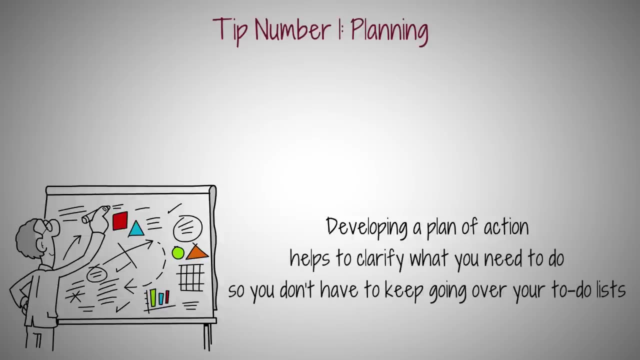 important to you. Let's look at five time management tips that can help you to work smart, not hard. Tip number one: planning. Developing a plan of action for your day, week or month helps to clarify what you need to do, so you don't have to keep going over your to-do lists. 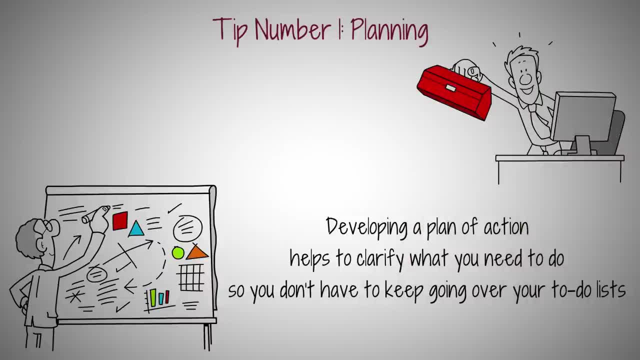 over and over again. One useful tool is called S-M-A-R-T- SMART. This acronym was developed by George T Doran, a consultant and director of corporate planning, in 1981 in Spokane, Washington. Although SMART does not have one definite meaning and has been revised over time to 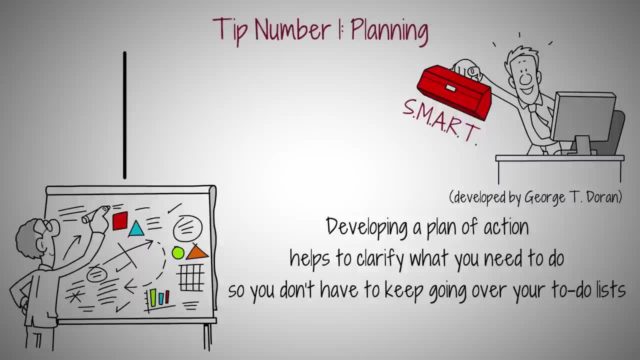 meet individual situations and needs. the original had five suggestions S Specific. Define a clear, specific goal. Know what it is you need to accomplish and what you need to accomplish M Measurable. Have some idea of how you will. 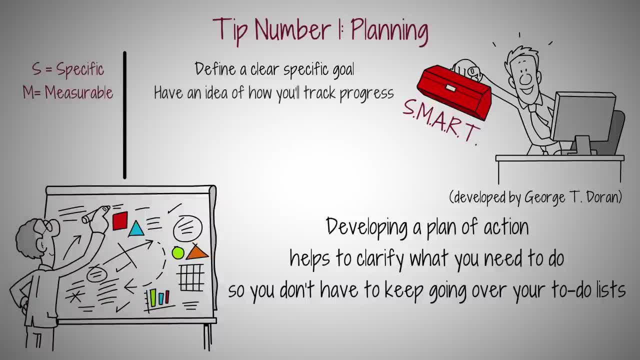 track your progress, Set a deadline or have a timer to show how long you have to accomplish this goal. A Assignable Decide who is going to do it. If you are working alone, then clearly the doer is you. If you are working with a team, 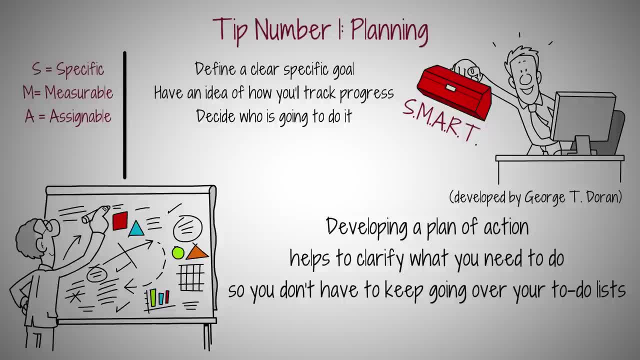 then be sure the person who is assigned the task is able and willing to complete it within the time frame specified. R- Realistic- Once you know what the goal is, you can start to plan ahead. If you know what the goal is and who is going to do it, be sure it can. 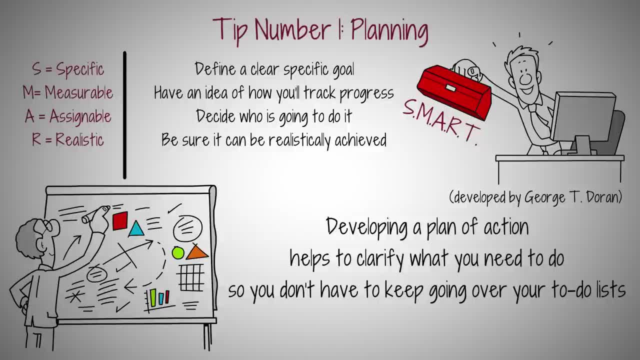 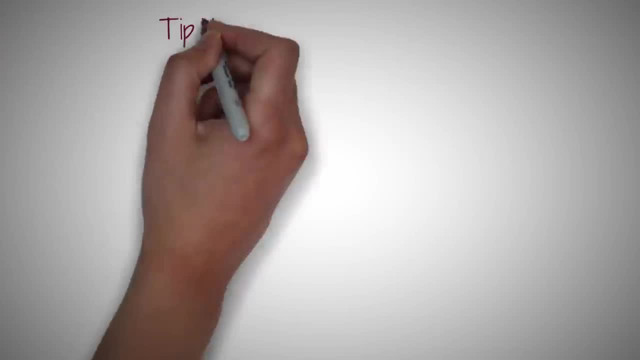 be realistically achieved within the time frame you have set and with the resources available. T Time: Assign a target date that is reasonable and attainable. Having a clear picture of what you want to get done clears the way to achieving it, Which leads us to the next tip. 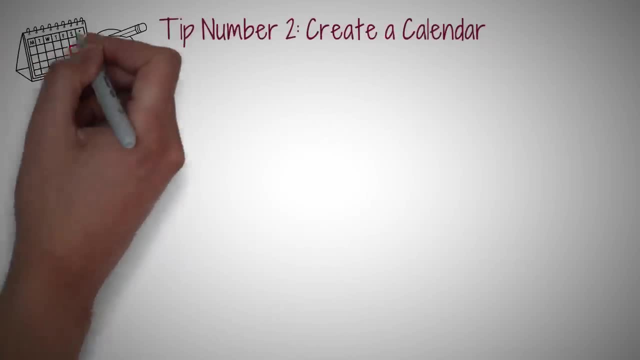 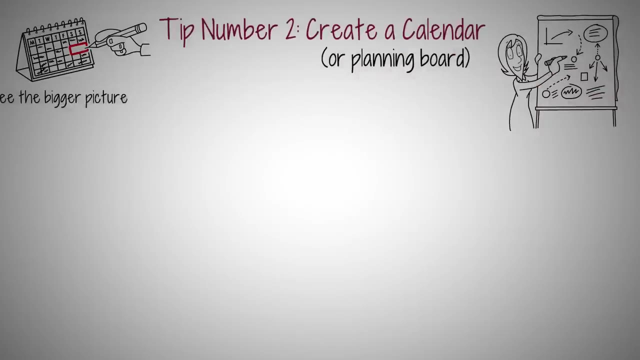 Tip number two: Create a calendar. Once you have a plan and you know what your tasks are that you want to complete, you can put them on a calendar or planning, a schedule or a planning board so you can see the bigger picture and assign a time frame to achieve. 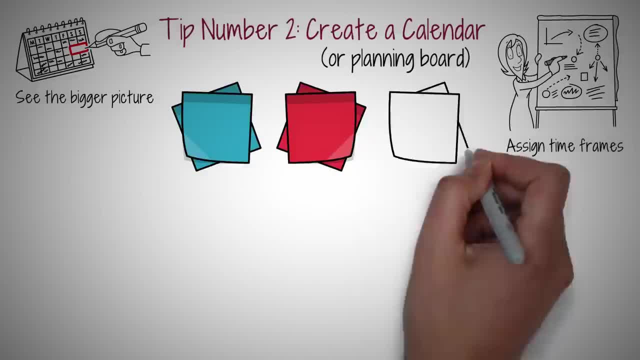 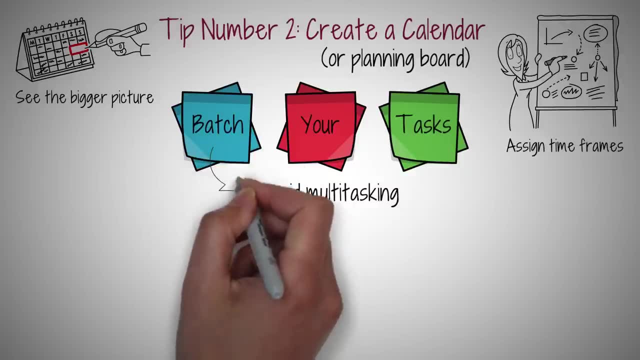 each job. By batching your tasks, you can group together similar topics, avoiding the energy-draining mode of multitasking. When you multitask, skipping from one unrelated job to another, it takes your brain some time to reset before you can become fully engaged in your project again. One study from the University of California: 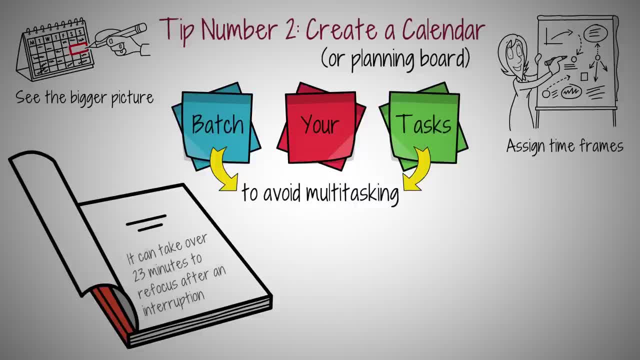 discovered that it can take over twenty-three minutes to refocus after an interruption. Imagine having to take twenty-three minutes out of every project just to get back in the flow of what you were thinking about. Use blocks of time containing similar tasks, like spending one hour in the morning and one hour at the end of the day to read and. 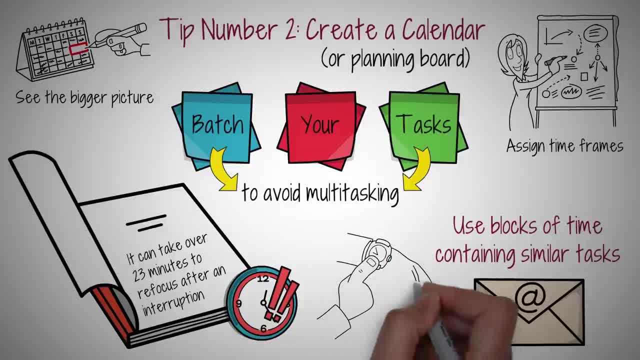 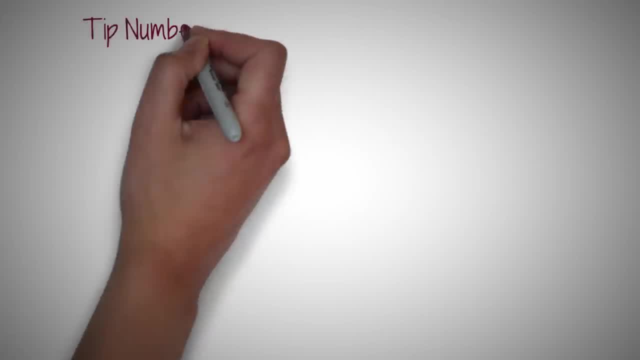 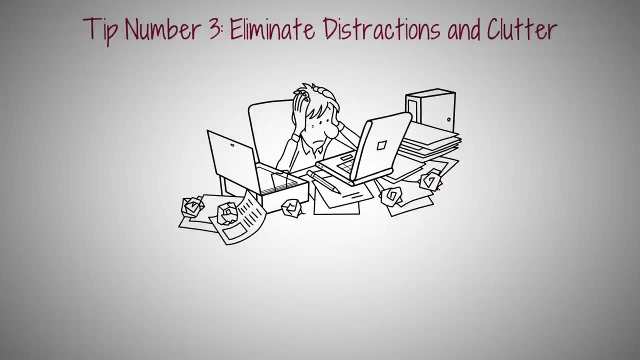 respond to emails. Then you can assign another group of similar tasks to another block of time. Think about one task at a time and focus on just that. Tip number three: Eliminate distractions and clutter. Keep your area clear of clutter. When you have piles of paperwork and too many objects in your 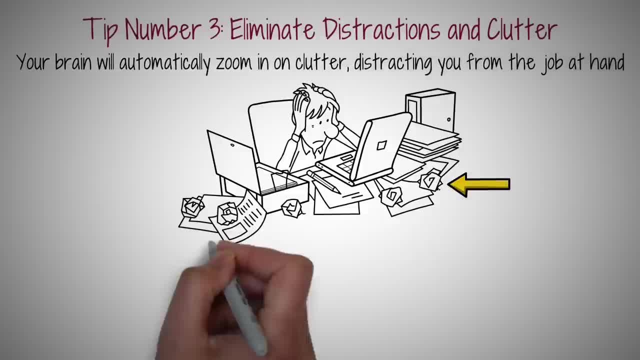 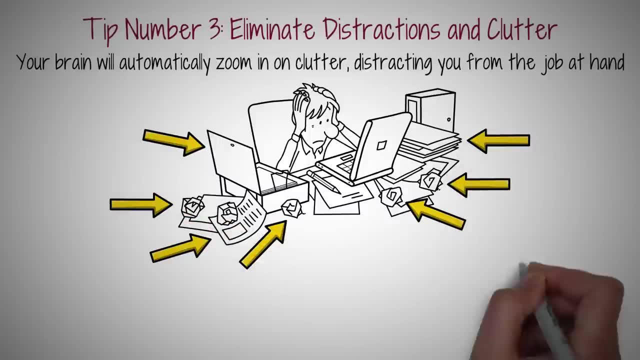 work area, your brain will automatically zoom in on them, distracting you from the job at hand. If you're looking at projects that are calling to you from the sidelines, you can be quite literally sidetracked from thinking about what you're doing now. By decluttering your work area, you can clear your mind and focus. 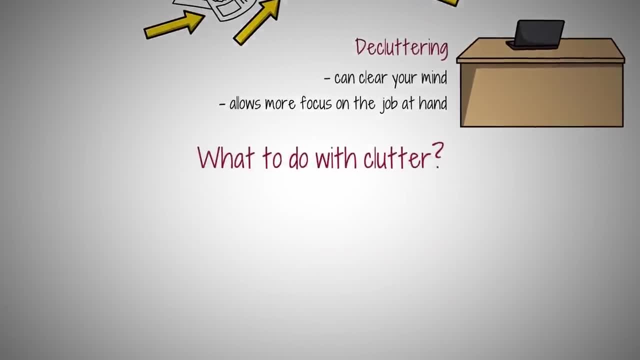 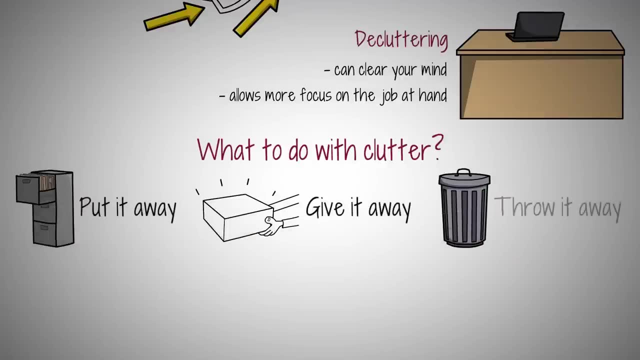 more on the job at hand. If you're having trouble deciding what to do with all of the materials on your desk, one rule of thumb could be to put it away, Give it away or throw it away. Most items will come under one of those categories. Putting. 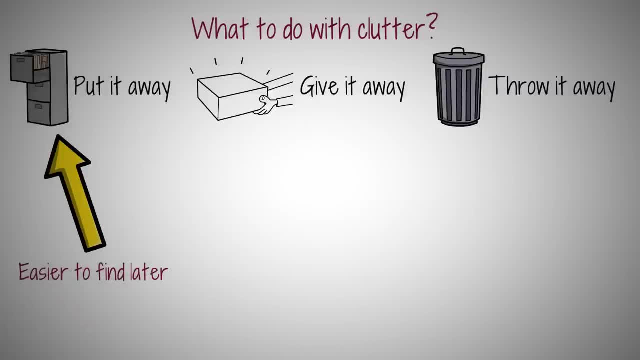 things away in an organized file, shelf or drawer will make it easier to find later, saving even more time, and it will be waiting for you when you are ready for it, not filling your head with all of the things you see needing attention on your desk, If it's something. 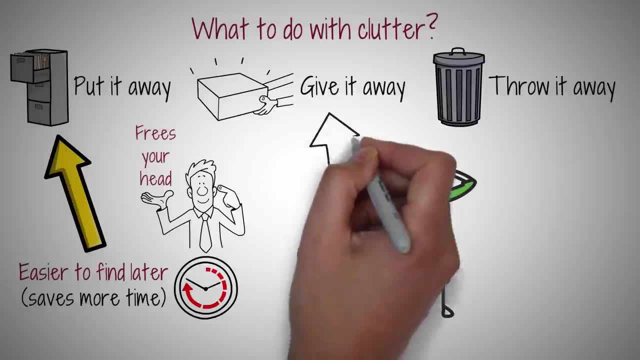 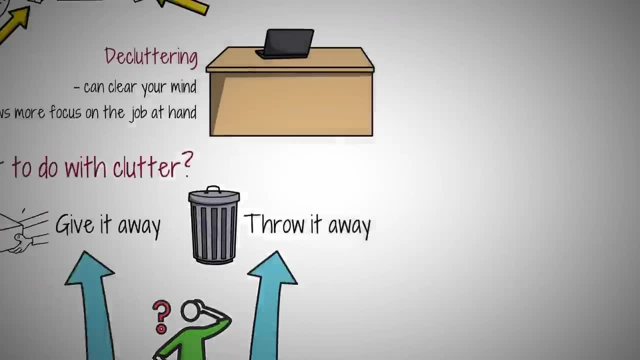 you no longer need. you can give it away to someone who can use it, or throw it away if it has no other purpose. If the assignment is going to be done by someone else, then for sure pass it their way. Tip number 4. Take breaks and drink water, While there's nothing wrong with working. 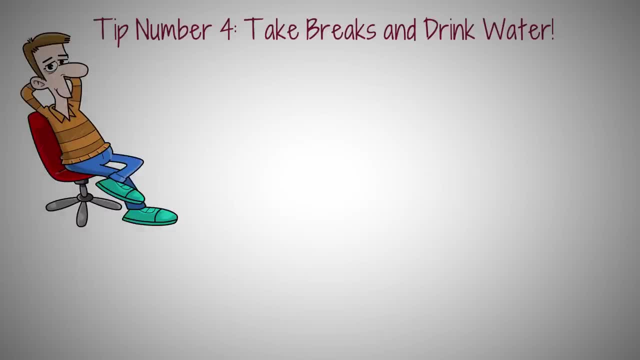 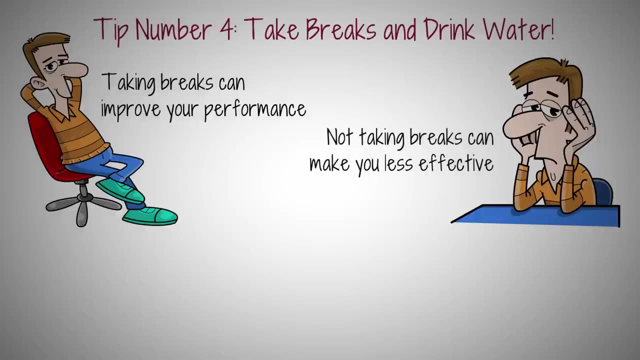 hard, especially when you are passionate about what you're doing. taking breaks can actually improve your performance. Not taking breaks can take its toll, making you less effective, not to mention the long-term effects on your body and mental health. Standing up and moving. 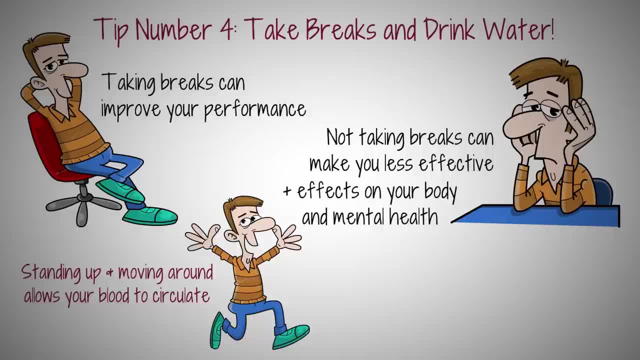 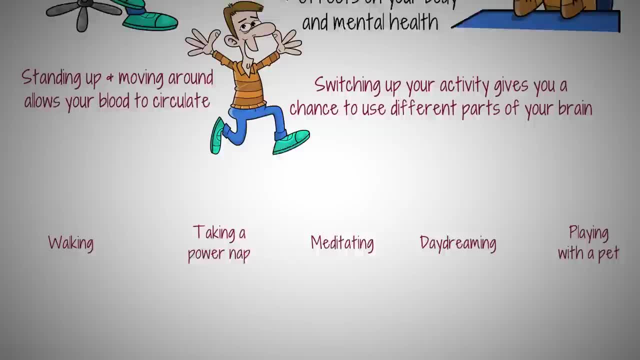 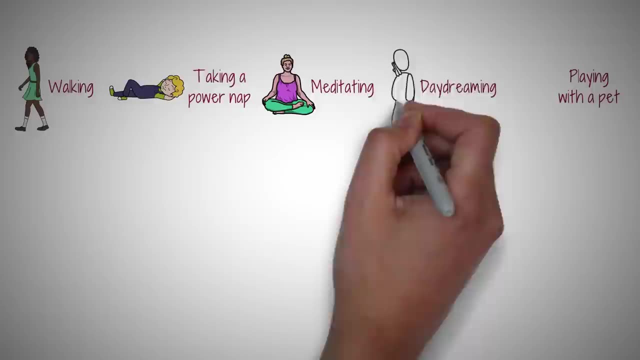 around allows your blood to circulate, and switching up your activity gives you a chance of your brain, rather than continual use of areas that control problem-solving, decision-making and even creativity. Walking, taking a power nap, meditating, daydreaming and playing. 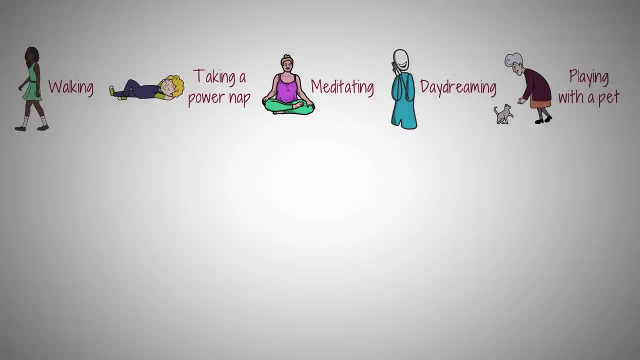 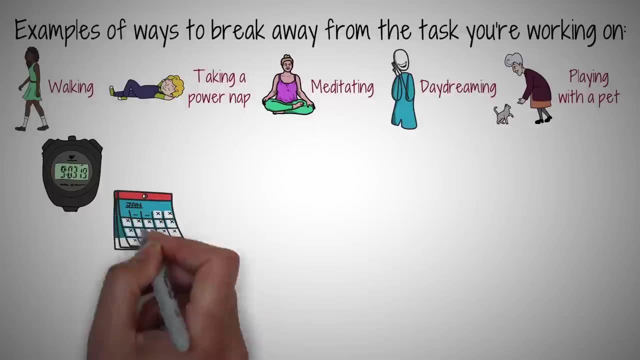 with a pet are all examples of ways to break away from the task you're working on. Set a timer to remind yourself to take time to do something different. You can even schedule it on your calendar, so you will have time set aside for it. Consider it another of your. 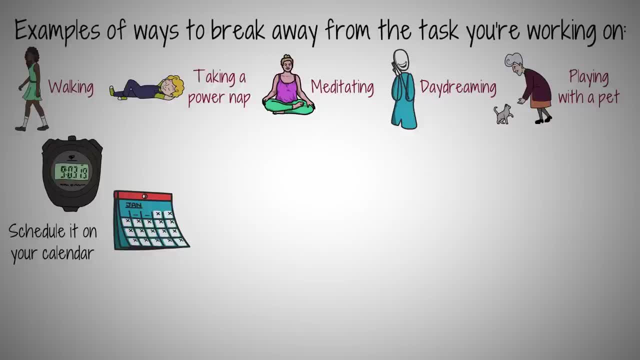 goals for the day, so you won't feel as though it's too late. Tip number 5. Take a break from your work and do something different, As though it's taking you away from your other tasks. it's just as important as all. 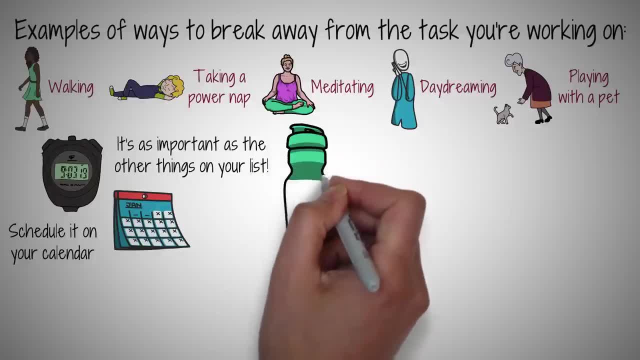 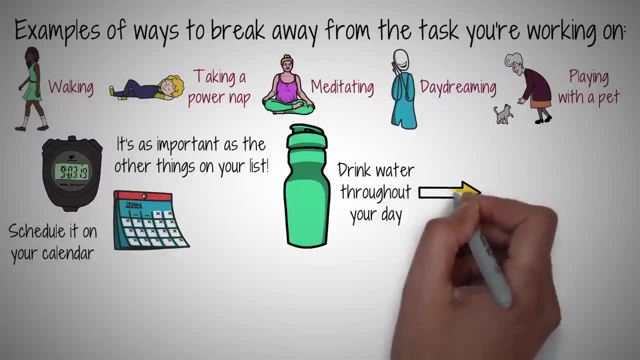 the other things on your list. While you're at it, remember to drink water either on your scheduled break or, better yet, throughout your day while you're working. Get your favorite water bottle or cup and keep it close by. Drinking plenty of water encourages brain. 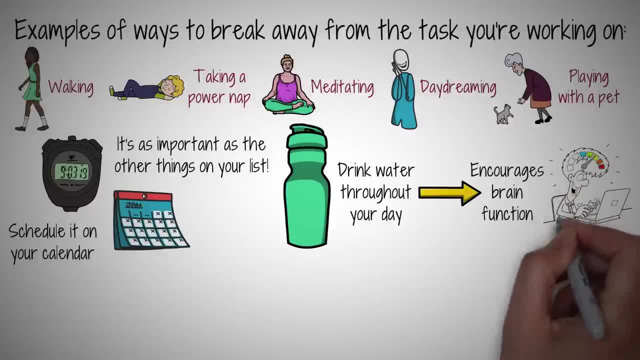 function. The human body is made up of over 50% water. after all, All of our cells and body systems need water to function at optimal levels. Tip number 6. Drink enough water to keep your brain functioning. When you are dehydrated, you might have a headache, feel sleepy or have lowered blood. 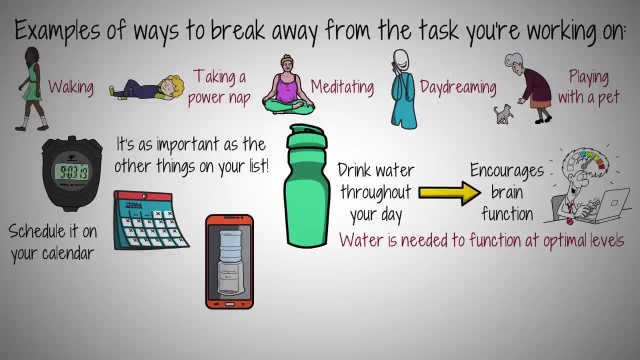 pressure—not the best situation for doing your best work. There are free apps like AquaAlert that can help you track your water intake and send you reminders that it's time to stop and rehydrate As you're putting your best foot forward to do your best at achieving 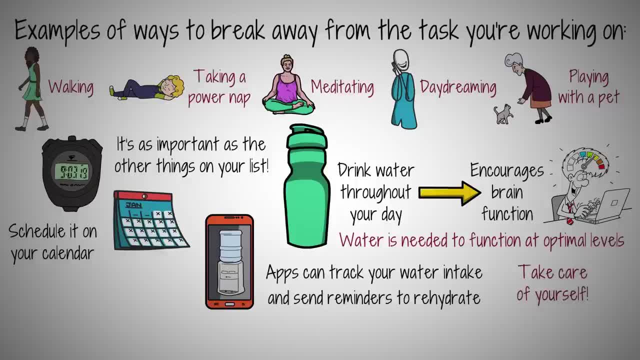 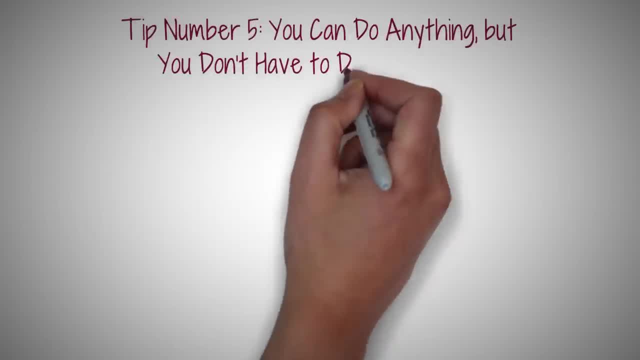 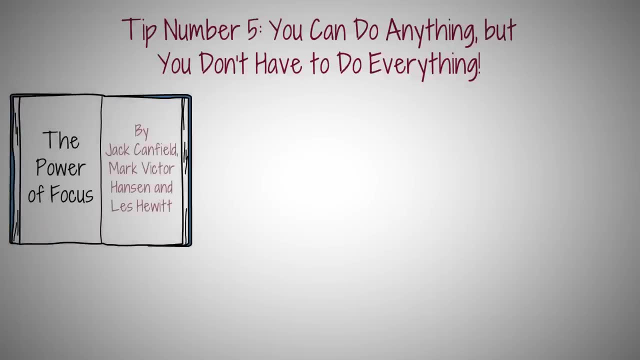 your work goals, remember to also take care of yourself. Your goals will not get far without you. Tip number 5. Use기를, and�ר can do anything, but you don't have to do everything. In a book called The Power of Focus by Jack Canfield, Mark Victor Hansen and Les Hewitt, 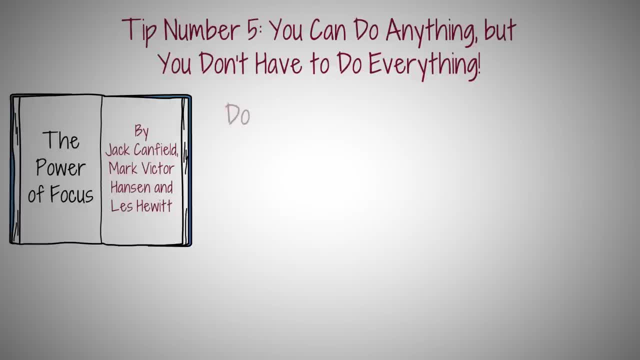 they describe the four Ds of time management. These are: Do, Defer, Delegate and Delete. In deciding what your goals are and how you're going to achieve them, it's helpful to prioritize the importance of each goal and how it will be carried out. 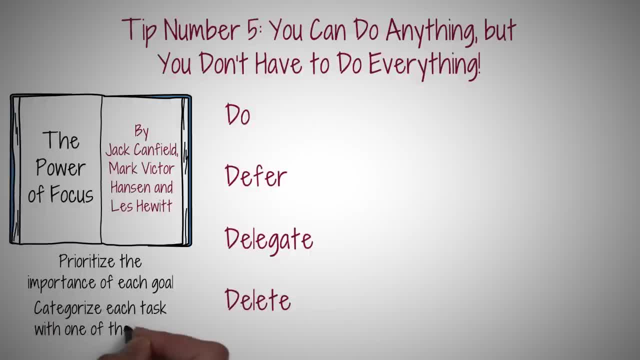 When looking over your list, categorize each task with one of the four Ds. If you choose to put it in your list as something to do, great, you've got it on your list. But if it seems like something that isn't urgent and you already have enough on your plate,